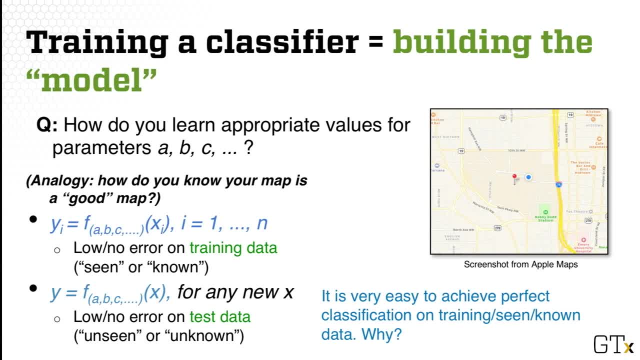 we want to know how to turn the knobs or the parameters in the model so that it can work really well for the training data, which is in other words for seen or known data where we train the model, or to build a model using those seen or known data. 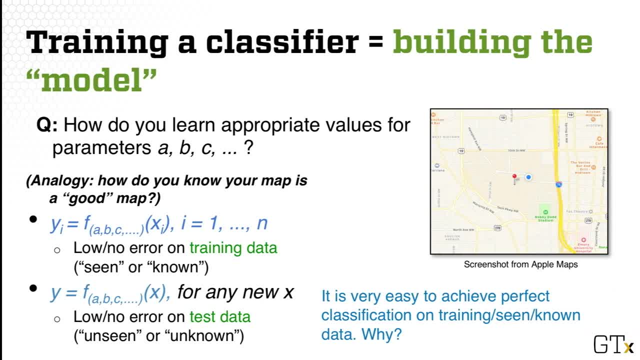 and we want the same model to work really well for the test data, which is, in other word, for unseen data, seen or unknown data, and training data and test data, or just a word, train and test in general is a very common terminology that you're going to hear a. 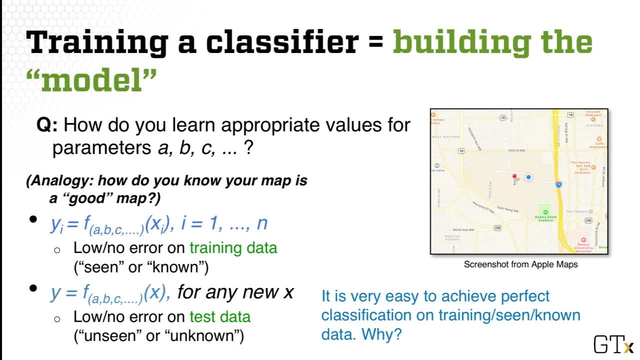 lot, so you may ask. so why do we really need to distinguish between training and test data? it seems like that I can. if I can get a very good model that works well for the training data, then it should ideally also work really well for the test or unknown data. so the main reason is that it's actually very easy. 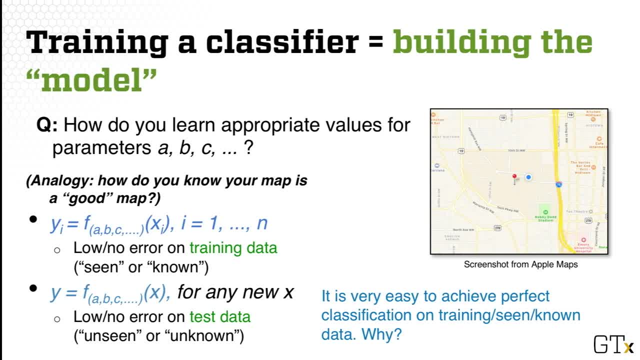 to have perfect classification on the training data. so that means you can actually build a perfect classification model that can have 100% accuracy. why can't it work so well and what's the problem with that? so the reason we can do it is because you can imagine, you can write millions of rules and that would 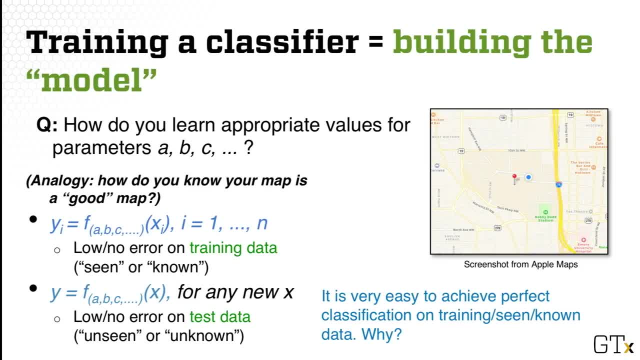 allow you to zero in to this very specific model and that would allow you to zero in to this very specific model and that would allow you to zero in to this very specific data point in your training specific data point in your training specific data point in your training data set. so that means, ideally, you can. 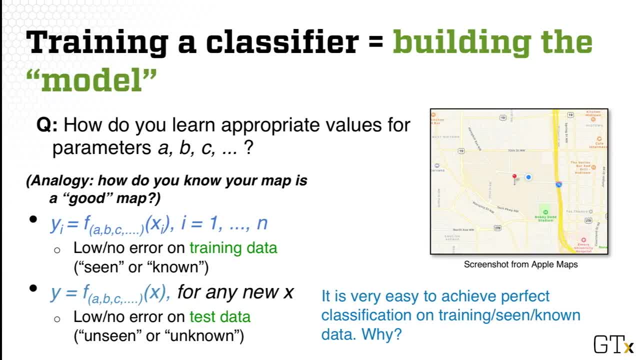 data set. so that means, ideally you can data set. so that means ideally you can just remember all the rules and then just remember all the rules, and then just remember all the rules and then also remember the label. so next time also remember the label. so next time. 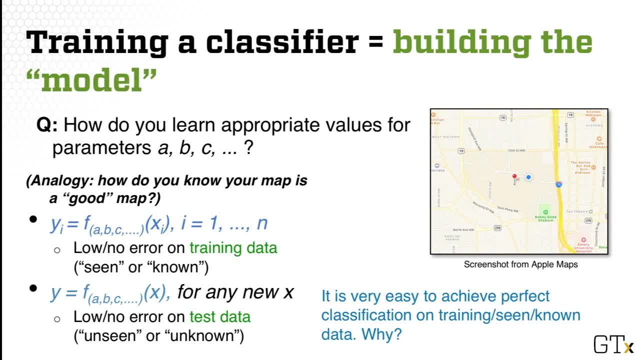 also remember the label. so next time, using other data points, that's exactly. using other data points, that's exactly. using other data points, that's exactly like your training data point. then you like your training data point, then you like your training data point. then you can just recall this, essentially like: 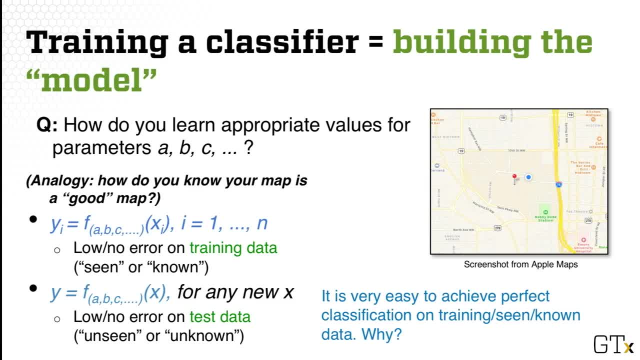 can just recall this essentially, like can just recall this essentially, like, looking up the labels, however, these looking up the labels, however, these looking up the labels, however, these millions of rules that you've written, millions of rules that you've written, millions of rules that you've written, they may actually not generalize to the 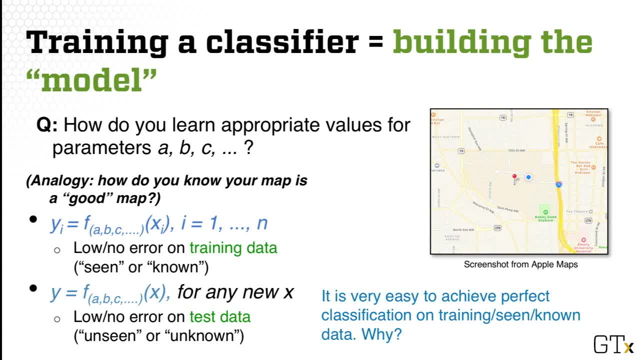 they may actually not generalize to the. they may actually not generalize to the. desk test data. so meaning you may have desk test data. so meaning you may have desk test data. so meaning you may have so many rules actually, you may not even so many rules. actually, you may not even. 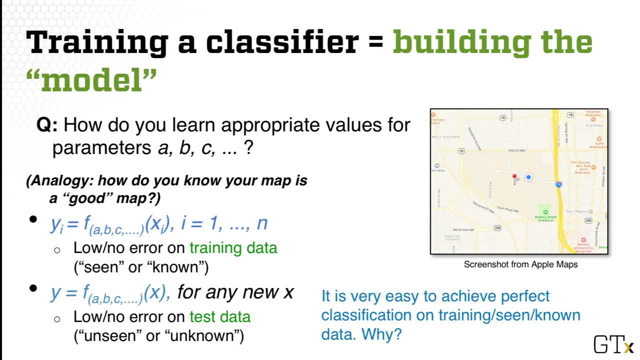 so many rules actually you may not even find any data points, that you have not find any data points, that you have not find any data points that you have not seen that that would fit those rules, so seen that that would fit those rules, so seen that that would fit those rules. so, when your model works really well for 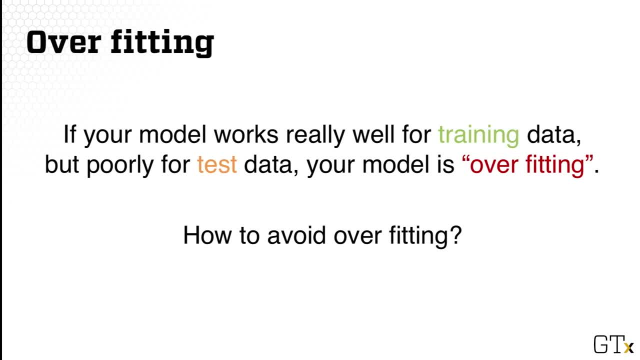 when your model works really well, for when your model works really well for training data, but very poorly for test training data, but very poorly for test training data, but very poorly for test data, then what we call is that your data. then what we call is that your. 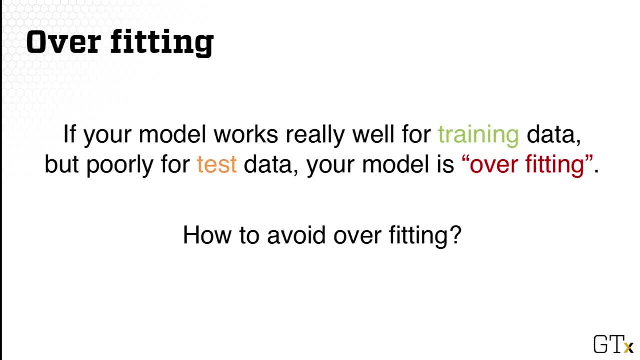 data, then what we call is that your model is overfitting. so this is the model is overfitting. so this is the model is overfitting. so this is the problem. obviously, because you ideally problem. obviously because you ideally problem. obviously because you ideally what you want is your model to work well. 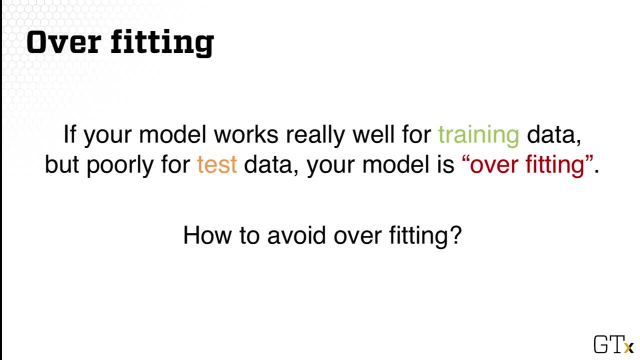 what you want is your model to work well. what you want is your model to work well for things that you don't know yet. so for things that you don't know yet. so for things that you don't know yet. so this is a prediction that all we care. 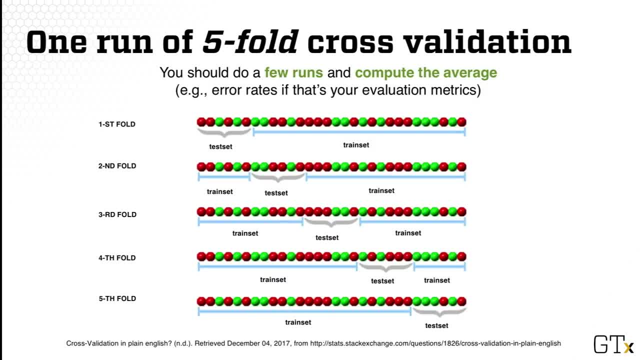 this is a prediction that all we care. this is a prediction that all we care about, so how do we avoid overfitting about? so? how do we avoid overfitting about? so? how do we avoid overfitting? cross-validation is a common technique. cross-validation is a common technique. 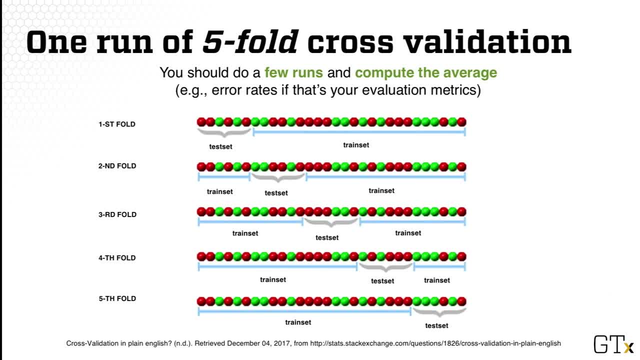 cross-validation is a common technique to prevent overfitting. so here we're to prevent overfitting. so here we're to prevent overfitting. so here we're looking at an example of how to do, looking at an example of how to do, looking at an example of how to do five-fold cross-validation, and 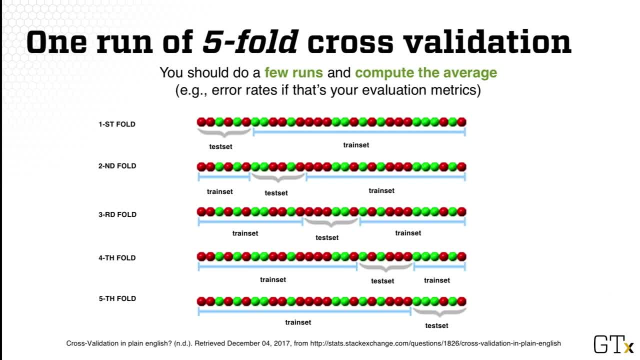 five-fold cross-validation and five-fold cross-validation, and specifically, we're looking at only one. specifically, we're looking at only one. specifically, we're looking at only one iteration of cross-validation. so in iteration of cross-validation, so in iteration of cross-validation, so in cross-validation, we will divide the data. 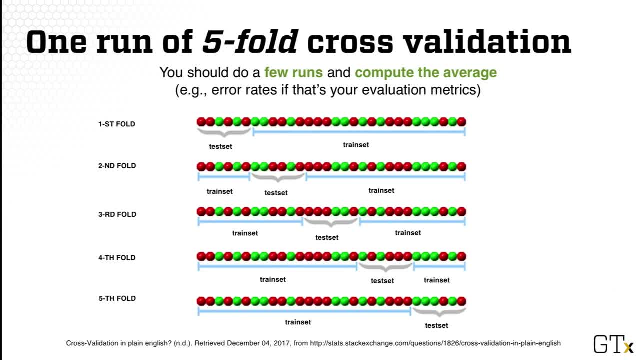 cross-validation. we will divide the data. cross-validation. we will divide the data into folds or parts, for example, in the. into folds or parts, for example, in the. into folds or parts. for example, in the first row. here you'll see that we. first row. here you'll see that we. 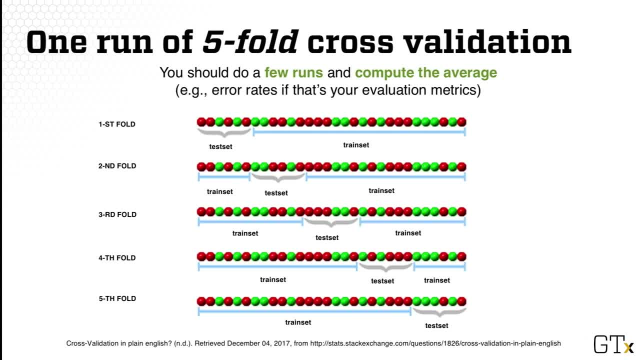 first row. here you'll see that we divided the data into five parts or five. divided the data into five parts or five. divided the data into five parts or five folds, and we'll use four folds or four folds. and we'll use four folds or four folds and we'll use four folds or four parts as a training data, which means: 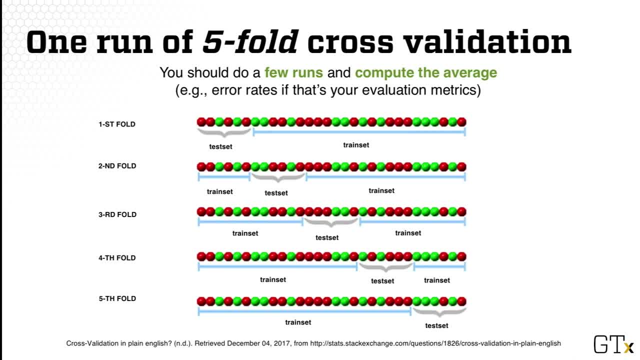 parts as a training data, which means parts as a training data, which means we're going to use these four parts to. we're going to use these four parts to. we're going to use these four parts to train or to build our model to figure. train or to build our model to figure. 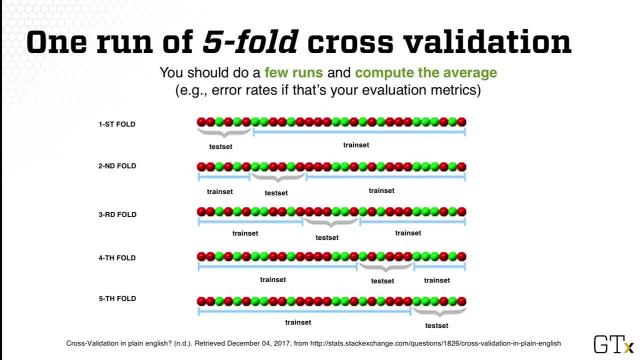 train or to build our model, to figure out its parameters. and once the model out its parameters, and once the model out its parameters, and once the model is built, then you, we evaluate it on the is built, then you, we evaluate it on the is built, then you, we evaluate it on the test set, which is a remaining part of 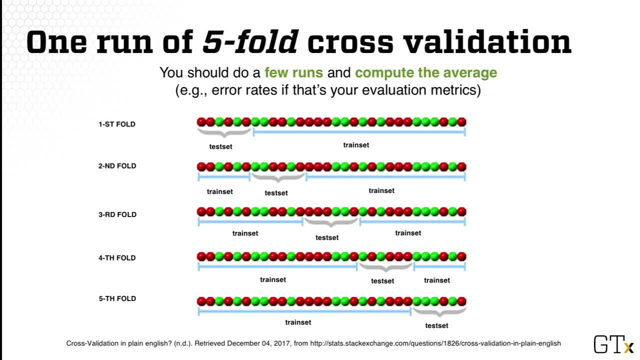 test set, which is a remaining part of test set, which is a remaining part of the remaining fold, and we'll get the, the remaining fold, and we'll get the, the remaining fold, and we'll get the accuracy for this fold, accuracy for this fold, accuracy for this fold, and we do the same thing for the second. 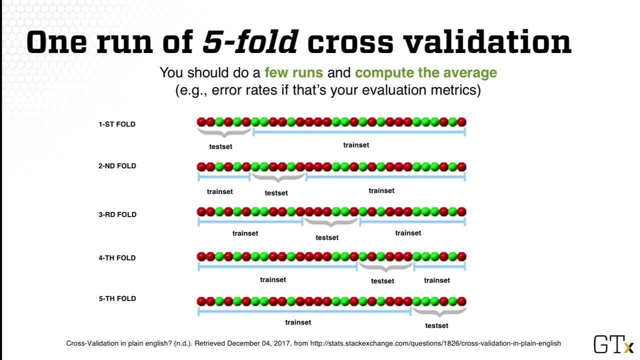 and we do the same thing for the second, and we do the same thing for the second: fold, fold, fold. so meaning we still use four parts as so meaning we still use four parts as so. meaning we still use four parts as training data set. but here you notice. 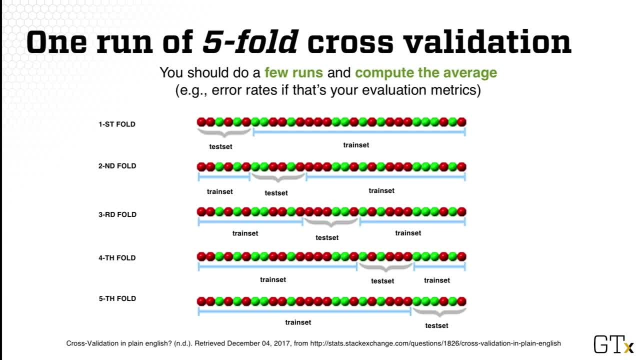 training data set. but here you notice training data set. but here you notice that we shift the test set to the second, that we shift the test set to the second, that we shift the test set to the second part, part, part, and again we get accuracy for this fold. 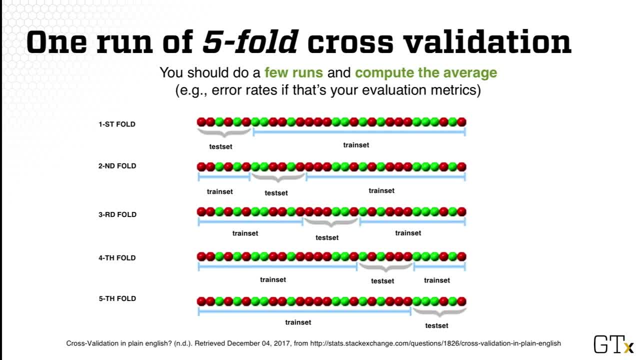 and again we get accuracy for this fold, And similarly we move to a third fold, and so on, And after doing all five folds, then we have five accuracies And what we do is to take the average. then that becomes our cross-solidation error. 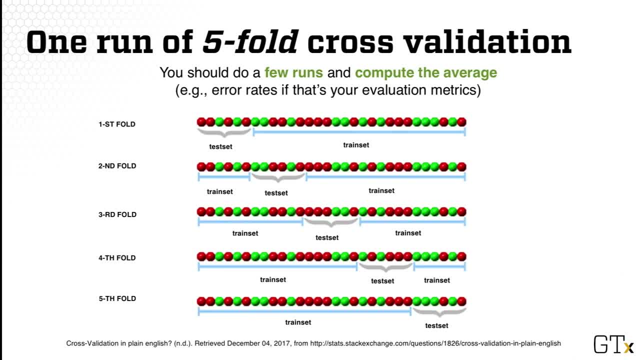 And of course, as we mentioned, this is only one iteration, So the accuracy that you get would depend on how you divide up the data. So that means ideally you want to do at least a few runs- The more runs the better- and to compute the average. 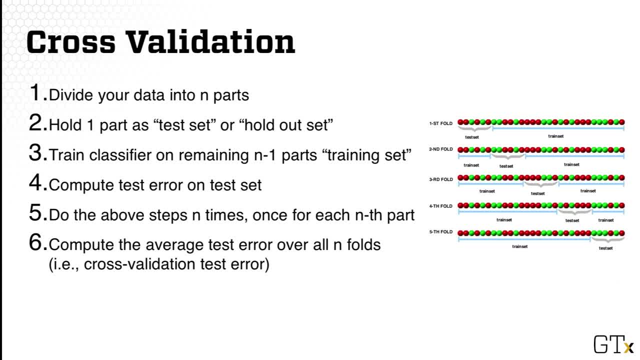 So, in other words, the exact steps that you need to do is to divide your data into n parts. You use one part as a test set or whole L set, and then you would train the data on the remaining n minus one part, what we call the training set. 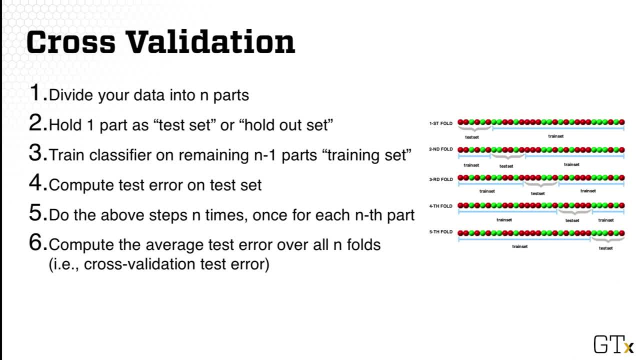 And after that we compute a test error on the test set. and we do step one to four n times, once for each of the n parts, And after that we compute the average test error over all folds. So when doing this, 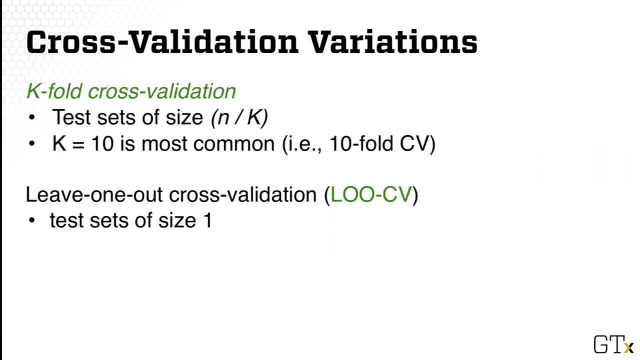 when doing cross-solidation we need to determine how many folds that we want to use, And the test set size of course depends on that number as well. So test set size equals the number of item n divided by the number of folds k. 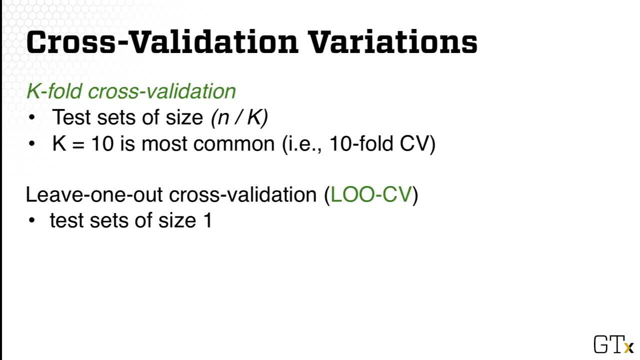 So k equals 10 is most common. So in other words, 10-fold cross-solidation is most common. There's a variation of cross-solidation called leaf one L cross-solidation, So it's a very fancy way to say essentially setting. 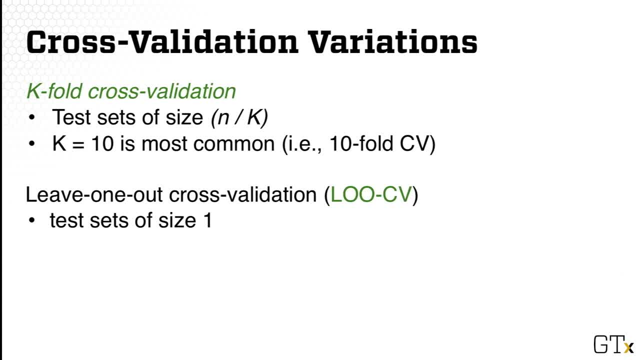 the number of folds that we want to use to divide the data into n parts or to the training, n times. So this is a great way, essentially using every single data point, to evaluate your model once, But, as you imagine, this is pretty expensive. 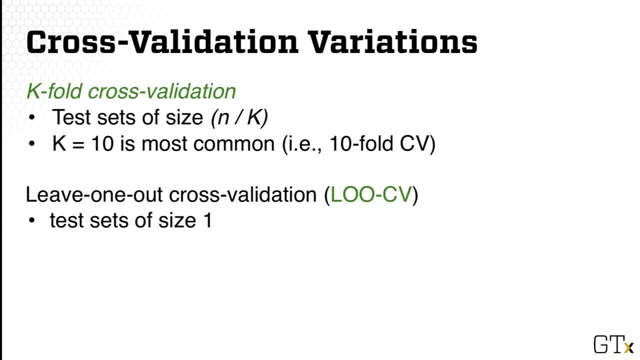 because you exactly need to divide the data into n parts or to the training n times. So often the recommended number to use is 10, because it's most common And using other numbers, generally we don't really recommend. For example, if you use k equals 9,.